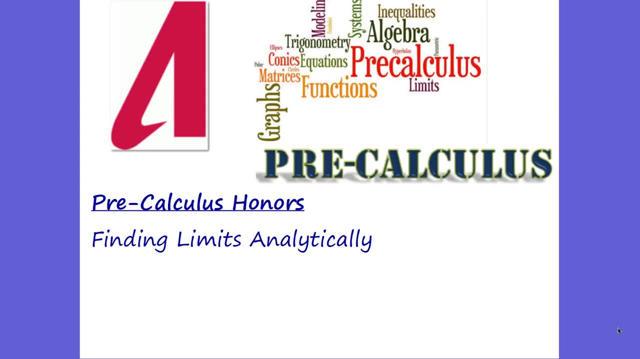 Hey, this is Mr Aiden. This is Pre-Calculus Honors and we are back in limits again and we're taking a look at finding limits analytically. We took a look last time how we found it using a table. We took a number really really close on the left hand side, really really close on the right hand side. We saw if they agreed. We took a look graphically whether the left hand side and the right hand side were able to agree. If they didn't, it did not exist, And so now we're going to take a look analytically, or what we call algebraically. The first type we're going to take a look at is 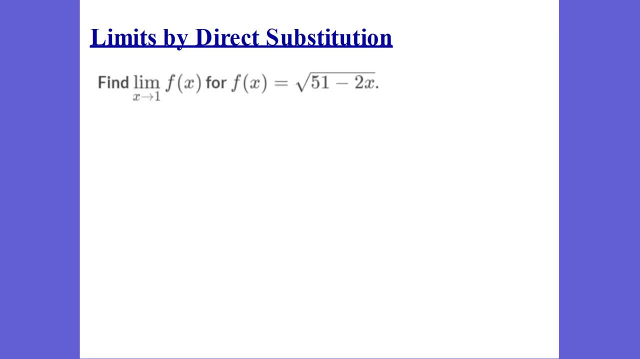 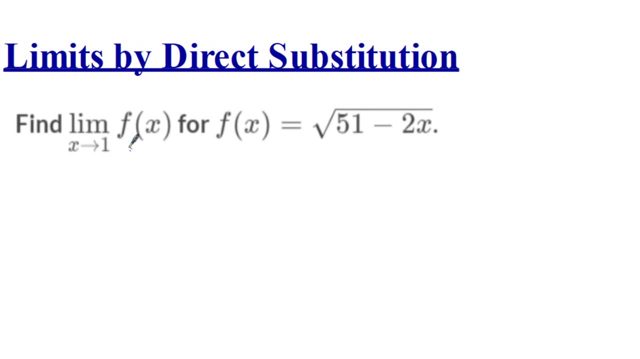 limits by direct substitution. Here we don't have a denominator that's going to cancel out, and we don't have a negative value, And so what we're going to do is we're going to take this limit as x approaches 1.. We're going to take this 1 and we're going to substitute right in for x, And so we have the square root of 51 minus 2 times 1.. And we know 2 times 1 is 2.. 51 minus 2 is 49.. And we have the square root of 49, which is equal to 7.. So that limit is 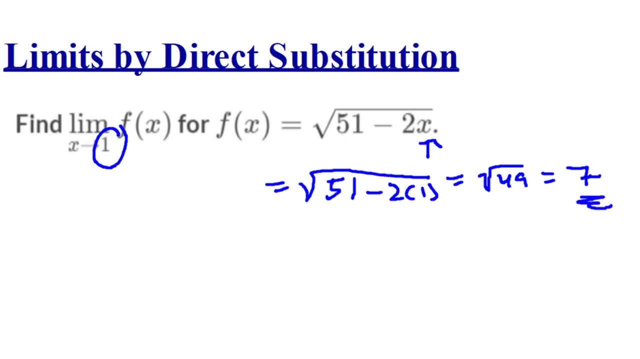 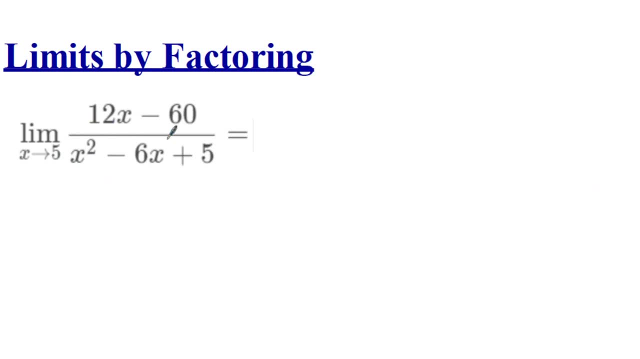 equal to 7. And that's using what we call direct substitution. Now we can also take a look at limits by factoring here. If we plug in 5, if we use direct substitution, we get 0 over 0. We get an indeterminate value, So we have to use it. looks like a little bit of factoring involved, And so we take a look at the numerator and we can factor out a 12 on that numerator, And so we have 12 and we have x minus 5 when we factor it out On the denominator. 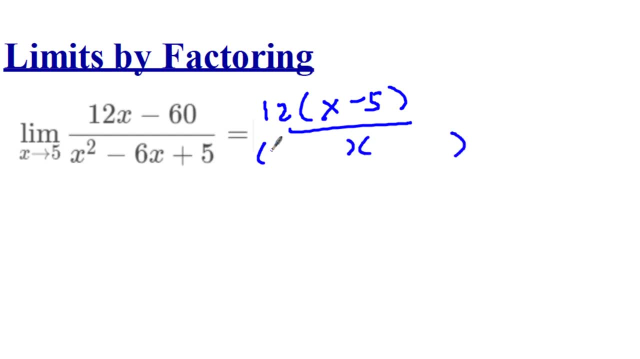 we can do our factoring. We can do: x squared is equal to x times x. We have our factors of positive 5 is negative 5 and negative 1, which add up to negative 6x. You can see what cancels out here is our negative 5s cancel out. We have a hole in that graph. So even though we have a hole in the graph does not mean that the limit does not exist, because even though there's a hole, it's not continuous. we still have a limit approaching from the left and the right hand side, And now we 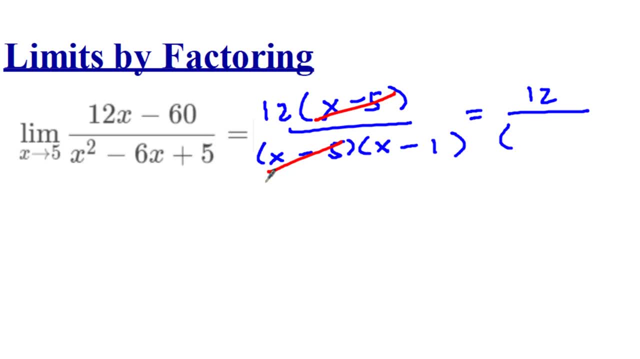 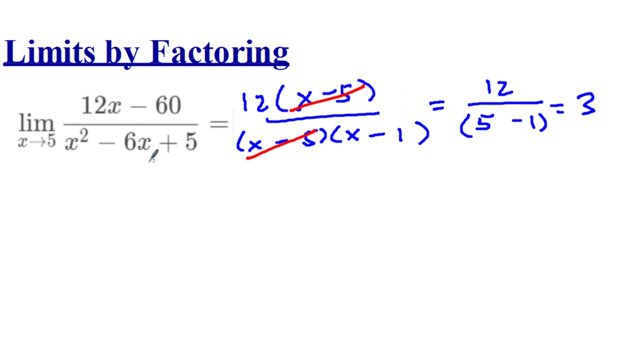 can use direct substitution. We have 12 on our numerator, We have x, which we're going to plug in our limit, as approaches 5 minus 1.. And we have 12 over 4, which is equal to a limit of 3.. So, even though that point is not defined, that limit does exist. That limit is equal to 3.. So we had limit by direct substitution, limits by factoring and our last is limits by using conjugates. 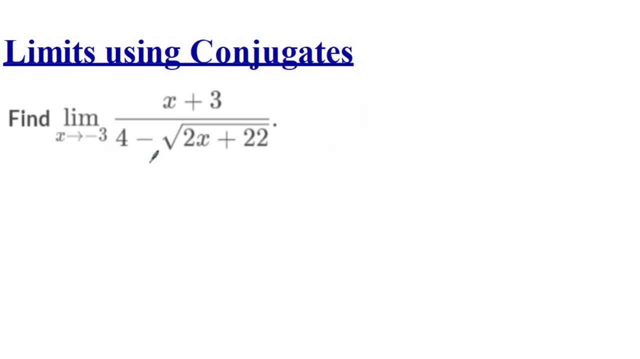 Again, if you put a negative 3 in here, we are going to get an undefined value. but that does not mean that the limit does not exist. And so in this type 1, we're going to multiply the top and bottom by the conjugate. We're going to multiply by 4 plus the square root of 2x plus 22.. On the bottom, we got to do the same thing to the top: 4 plus the square root of 2x plus 22.. And so whenever I use conjugates, 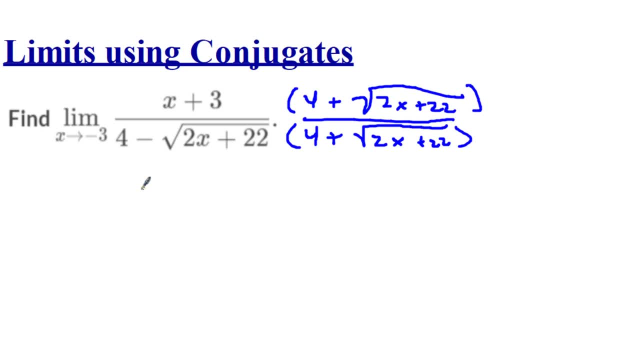 don't distribute that numerator. Or if it's on the denominator, what you multiply by, don't distribute it. So you keep your x plus 3 there, Keep your 4 plus the square root of 2x plus 22.. You're going to see why we don't want to distribute that. On the bottom we have to do some foiling So we have 4 times 4, which is 16.. Since we multiply by the conjugate that negative and that positive, that middle number is going to cancel out, But the bottom is going to be minus. 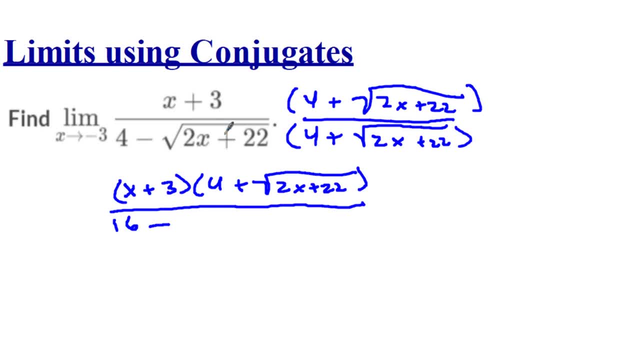 2x plus 22, because the square root of 2x plus 22 times the square root of 2x plus 22 equals 2x plus 22.. Watch out, That negative is going to distribute to everything on the denominator. And so on our numerator, we still have x plus 3.. We have 4 plus the square root of 2x plus 22.. On our denominator, we have 16 minus 2x minus 22,, which when